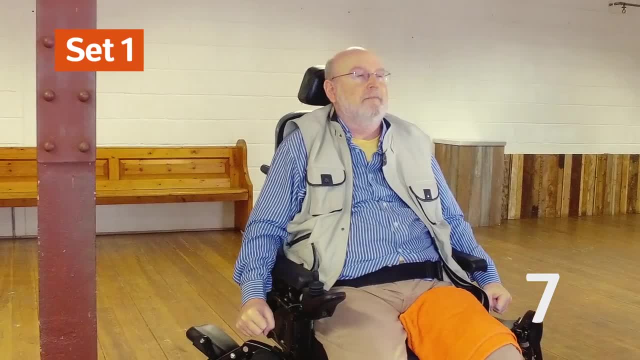 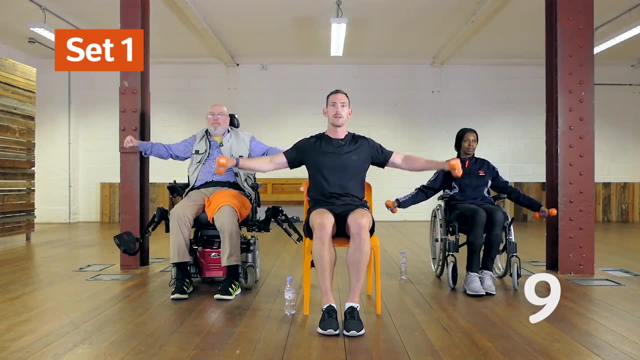 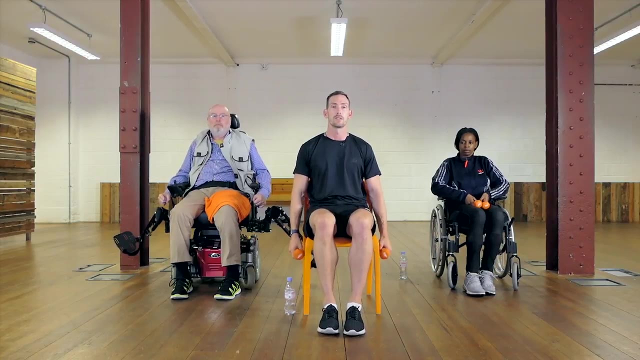 go crazy. Okay, three more to go, and then last one, up we come and go down, Okay. so give a chance to give your shoulders a little bit of a break, because this is quite a shoulder heavy exercise. So back onto the front. raises Three, two, one and. 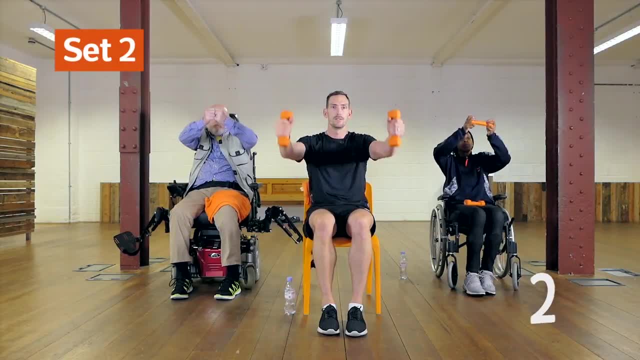 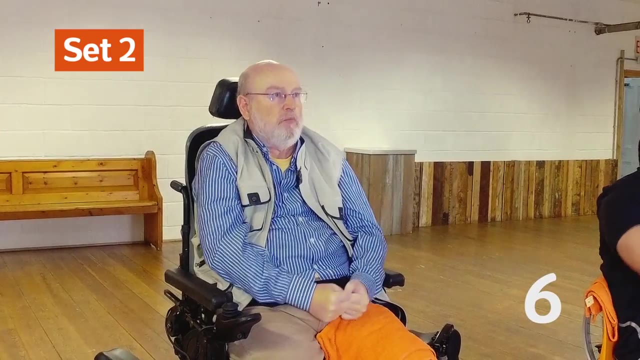 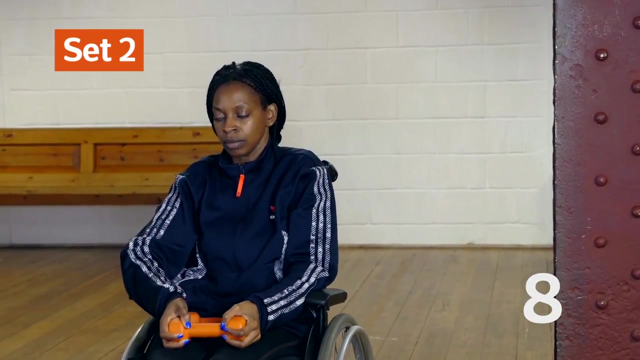 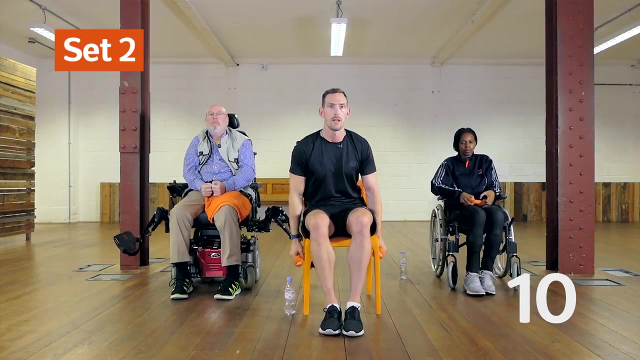 let's go One, two lovely stuff, guys, Three down, keep pushing, doing really well. That's five, halfway Seven. that's three left Nine, and then one more after this: Ten, ten great stuff. Okay, we have another moment to get a second dumbbell and then lateral. 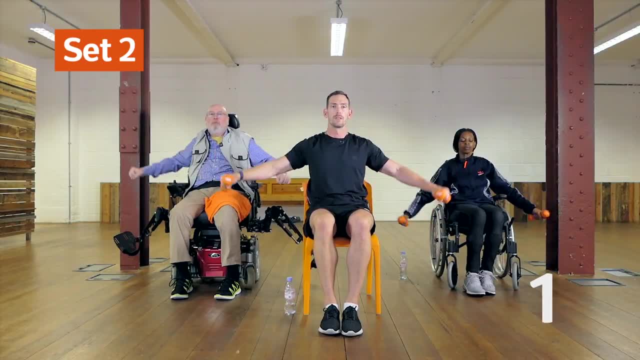 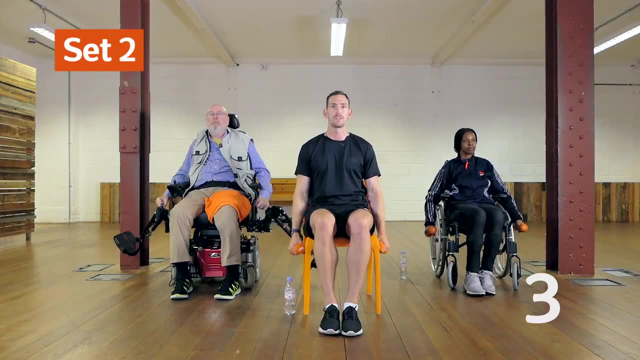 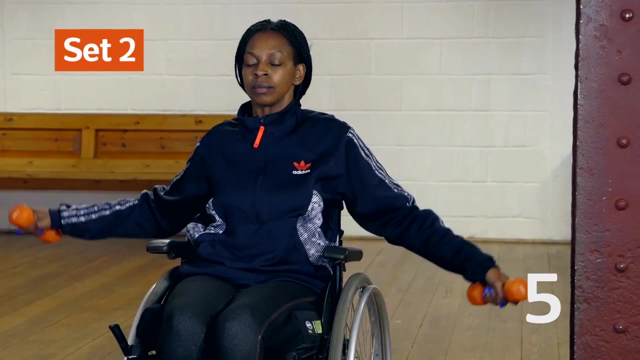 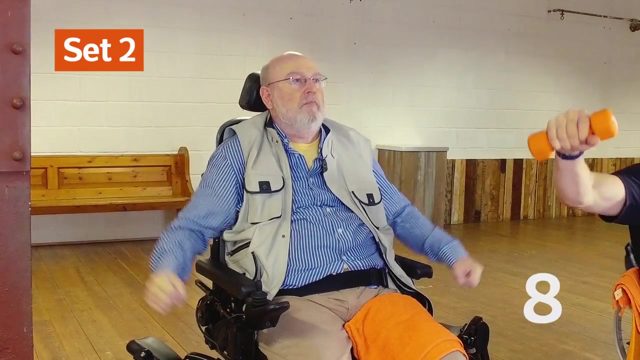 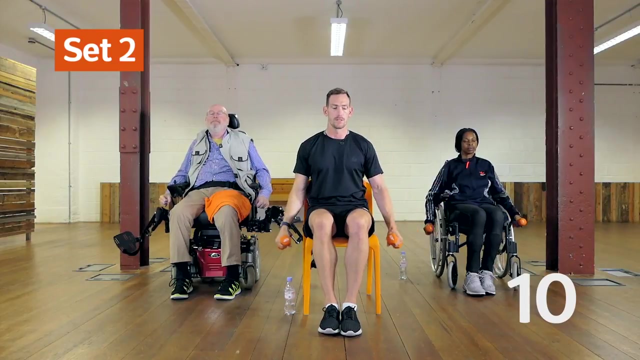 raises Three, two, one off, we go. Excellent stuff. Three down, seven to go. That's your halfway point right there. keep it going. Five more And last three, And then one more time. Good, Two sets of ten done. So we've got the final set for. 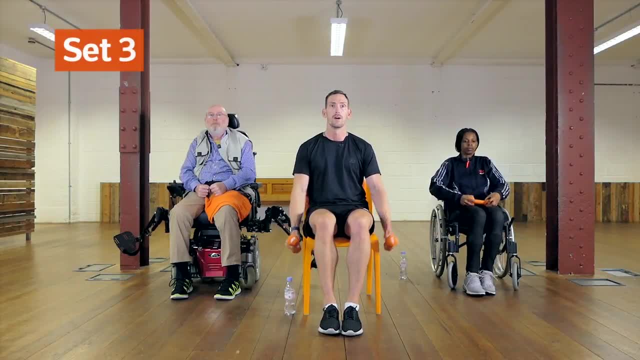 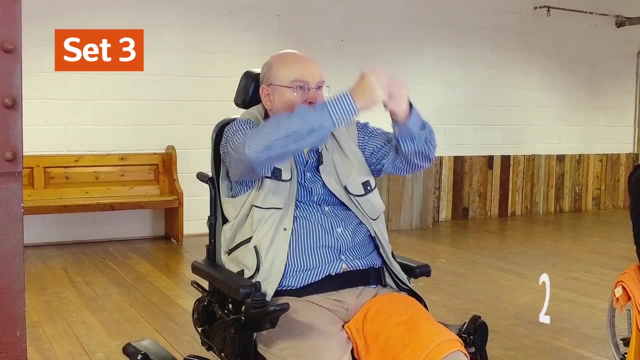 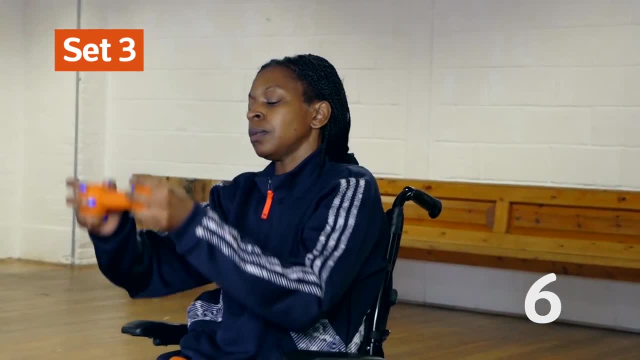 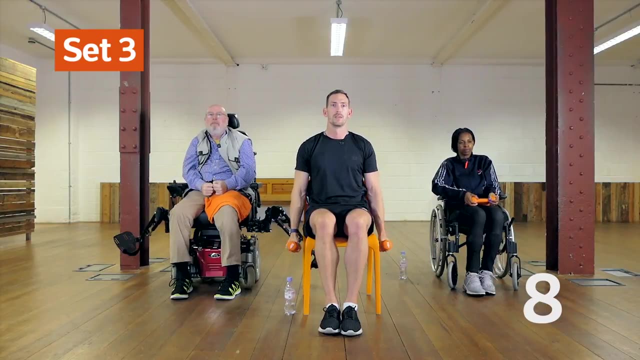 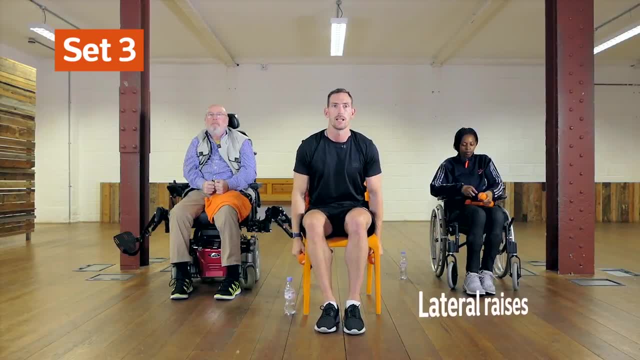 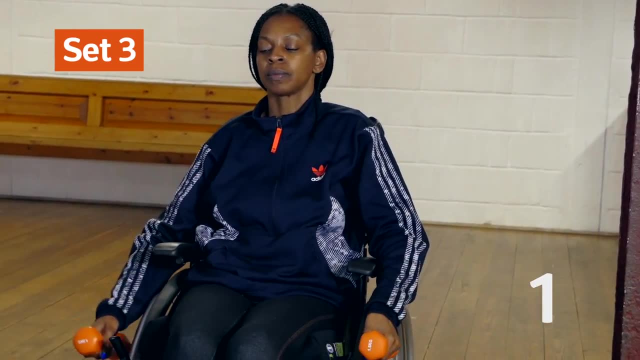 Good, nearly there. Last three exercises: Three, two, one. and okay, We've got just the last exercise, the lateral raise. So when you're ready with both Three, two, one, off we go. That's it.